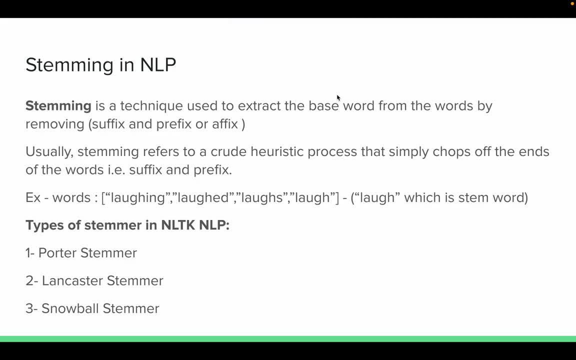 Hello everyone. So welcome back to our channel, that is, AI Next Generation. So today topic will be related to the stemming in the NLP. So you already have seen in the previous video that is related to the text preprocessing step, or whether which particular you have to use, how to substitute that particular with the help of regular expression. You have done the text preprocessing step part. So now come this: what we are just going to use, the stemming. Stemming is basically a. 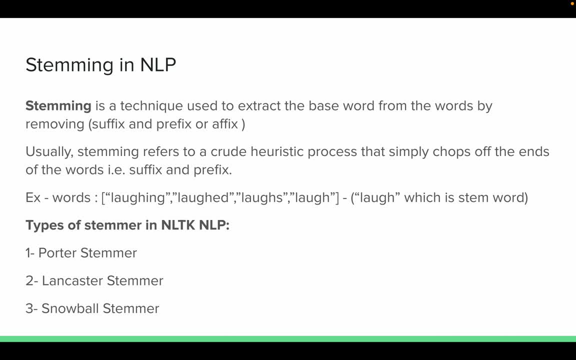 text normalization part. So text normalization means you are you here, you can use stemming or you can use limitization. So two type of technique we are going to deal with the natural language processing. The first we will understand in this video, that is just stemming, Stemming in natural language processing. So what is stemming? So stemming is basically used for the text normalization. So why? So stemming is a technique used to extract the base word from the word. So first of all, I will 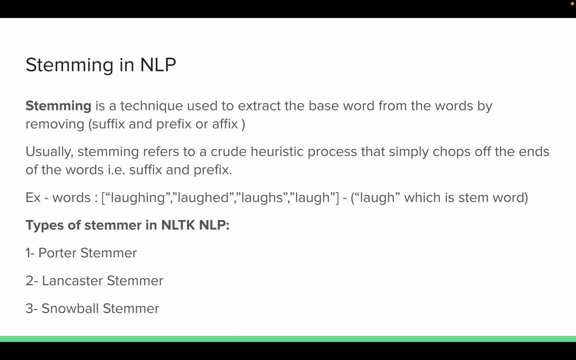 just give you the example So you will be able to understand more clearly. Suppose you have in one particular sentence you have text, or you have words, documents, In that particular one sentence, you will have laughing words. In the second sentence you will have the laughed and laughs. So what are these four particular words? What are the root word or base word for that? That is a laugh. So this is the root word, Even if you take an example of walking, walk, walk. The root word. 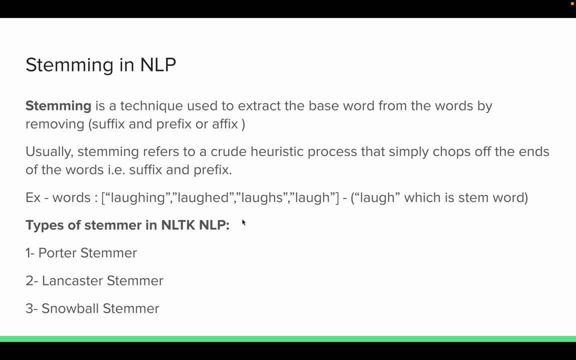 we walk. okay, so that's how you have to do, for the stemming means you want to extract from the words, that is, you have to accept the base word from the words. okay, so this is the main purpose of the stemming. okay, so even we will see in the practical part how we are going to use this. 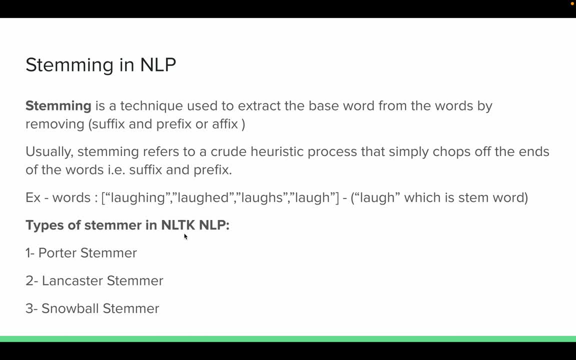 stemming and how, which. there are various type of technique to use the stemming. okay, so usually, first of all, usually, stemming refer to a crude heretical process. okay, that simply means it's shop of the ends of the words. okay, that is a suffix of the prefix. okay, it's simply saying: 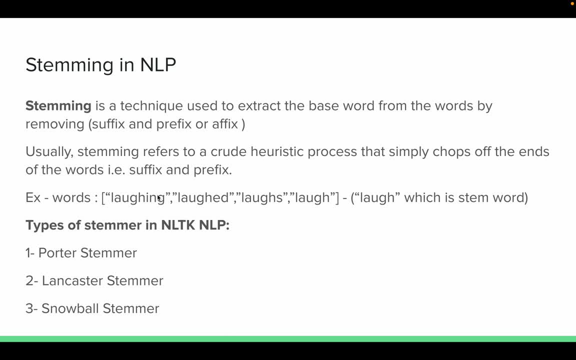 that whenever you are using laughing or love, it's directly chop of the ing. here is shop of the ad. okay, so this how the stemming works. okay, so stemming basically, uh, there are three type of stemming we are going to see in nltk library. that is one you will see: the portal streamer. okay then, 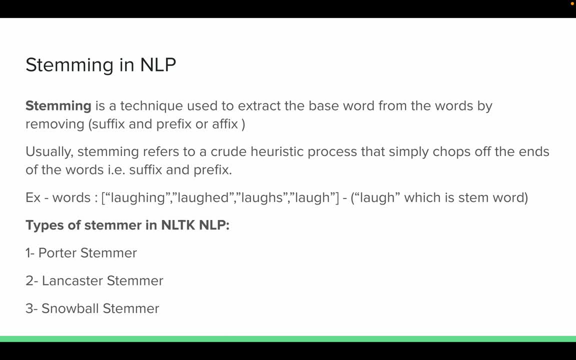 after you will see the lanchester streamer and then after you will see the snowball streamer. okay, so this, all three we will implement in this particular library in this google collab so you will able to see how we are just doing and how we it is. 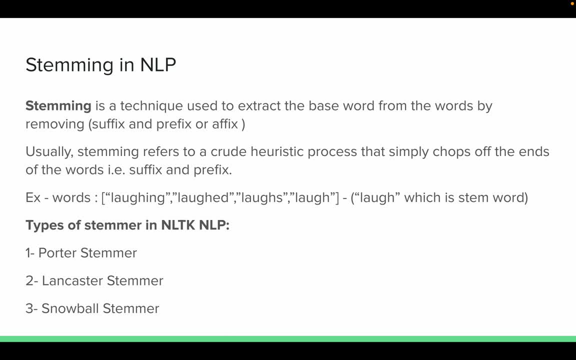 working in the case of this. all three technique. okay, so i think hope you understand the basic concept of the stemming, that is, the three part. it is clear to you that that is. stemming is basically to extract the base word or root word from the words. okay, so now let's jump to the coding part. 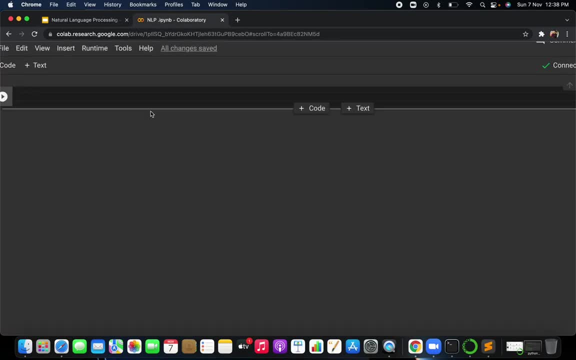 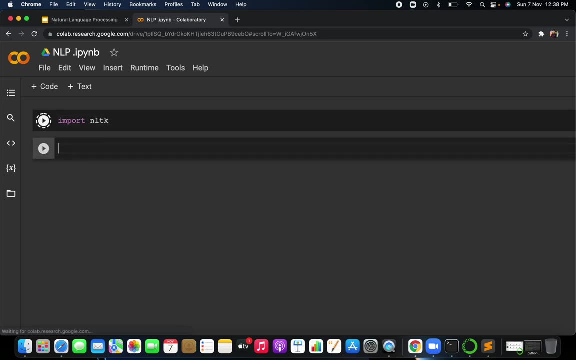 okay, first of all, before starting, we have to just load the basically analytical library. okay, you can just import, import nlt. okay, that's it. then. after that, what you have to just read, the first uh technique we are going to use, that is a portal streamer. okay, then, for the portrait streamer, what you have to just write here: 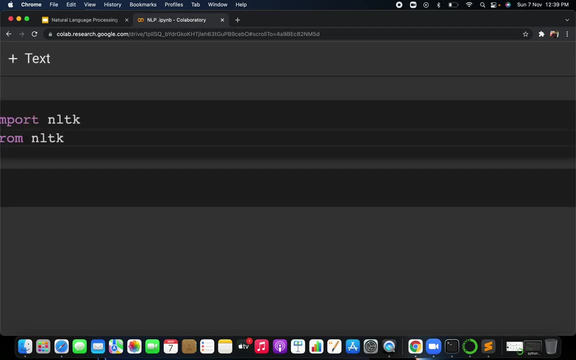 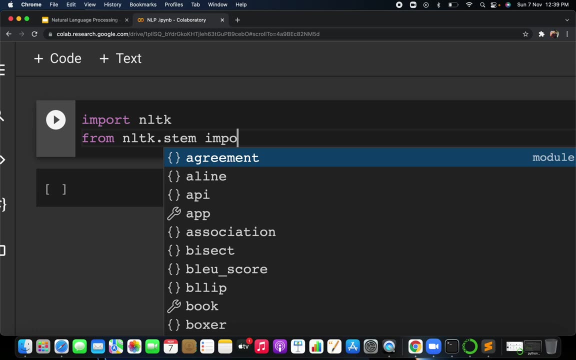 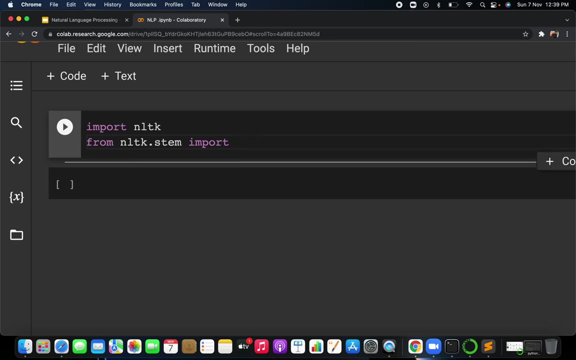 just write from nltk. you can just see: from nltk dot stem, okay. so from nltk dot stem. you want portals, streamer- okay, you can just write porter. streamer, okay, quarter. and then after you can just write streamer, okay, you can just run this thing. i hope so it will run okay. then after that just make the object of. 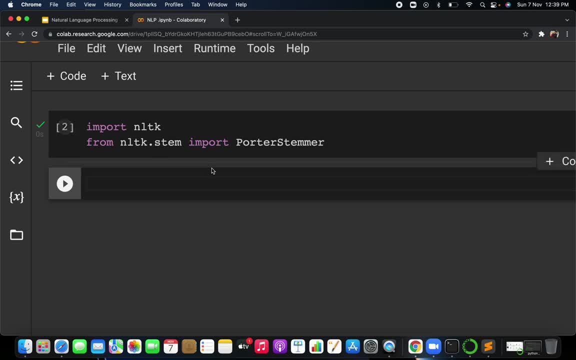 this particular method. okay, how you can just do. you can just write ps equal to quarter. then after streamer, okay, just make the object of that, that's it. then after that, you, you want to see how they are. just, uh, potter streamer is behaving already. we have seen the example in the slides, where i 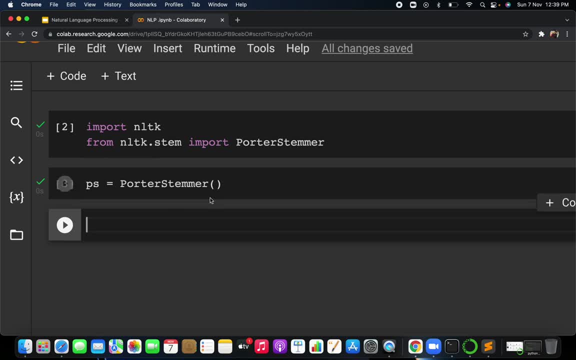 have shown you about the laughing, laugh and laugh. so we will use this particle portal streamer, so that particular words: okay, and how you will do. just write reporters. if yes, already you have, you can do it. okay from psstem. just call this particular method and just pass which particular. 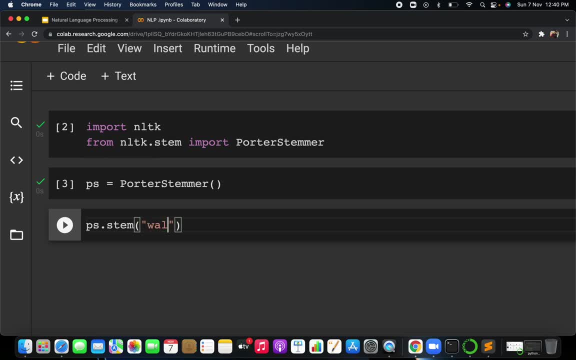 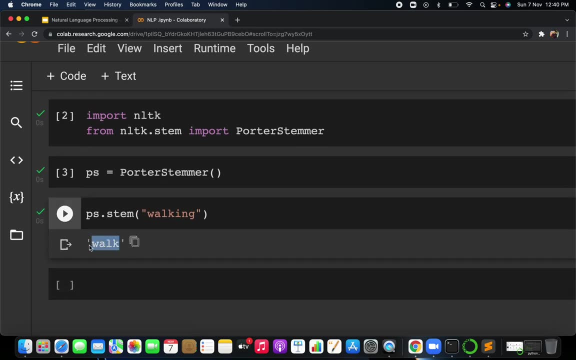 thing you want to do, okay, okay. so first of all, if i'm just doing for the walking already we have seen for the laughing- then you can just show for the how walking it is. see, this is the root word. okay, so you are just getting the root word from this particular walking, okay, so if i'm just saying 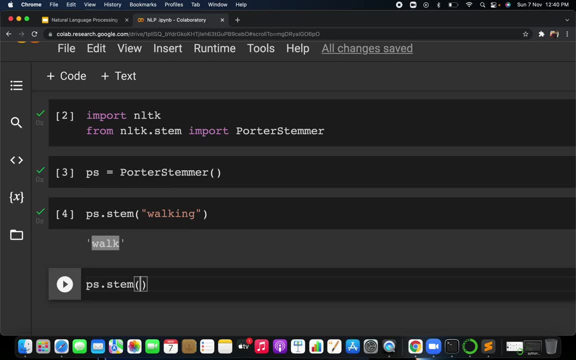 basically, if ps dot stem, i'm not going to say this is this particular one. i'm going to say if ps dot just saying and laughing, okay, i'm just, uh, not laughing, we can just concentrate with the walk. okay, i'm saying walked, okay, like random, i'm just taking. okay, see here it is also it's giving the. 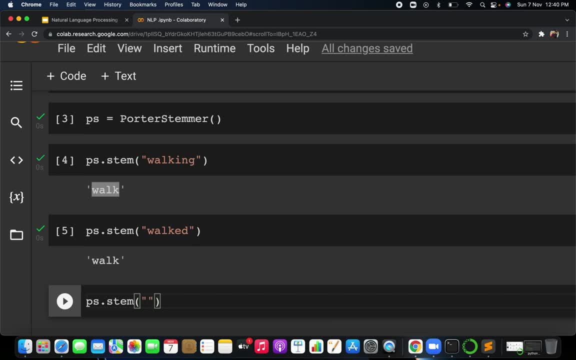 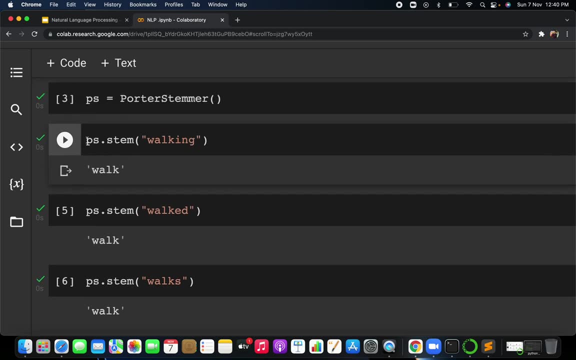 roots word and after, if you are going for, uh, just writing walks, okay, this what you are just writing. so i think it's clear. you are just getting the root word from this particular portal streamer. you are using the portal streamer technique of that particular stemming in analytical library. 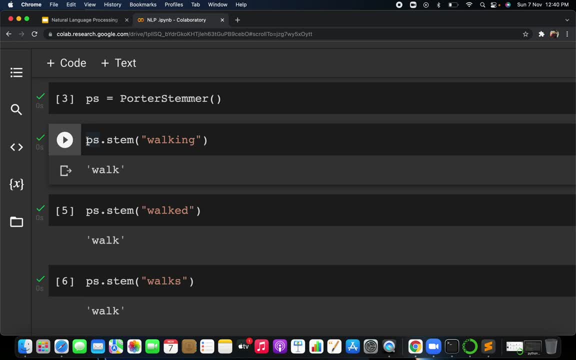 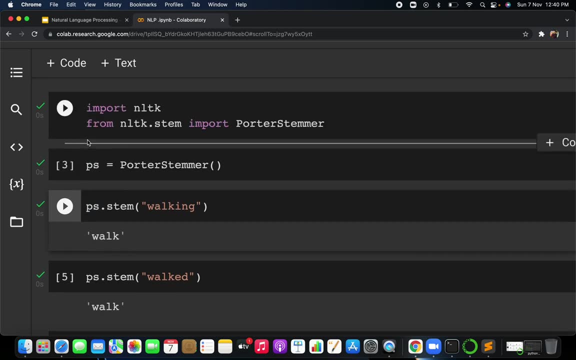 and this from here. you are just getting the root word from this particular words. okay, so i think it is clear to you about the how the protest streamer you are going to use: okay, the first we are going to use that is a portal streamer. okay, then after that you are going. 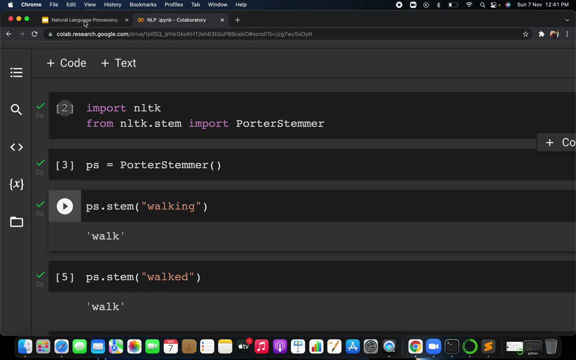 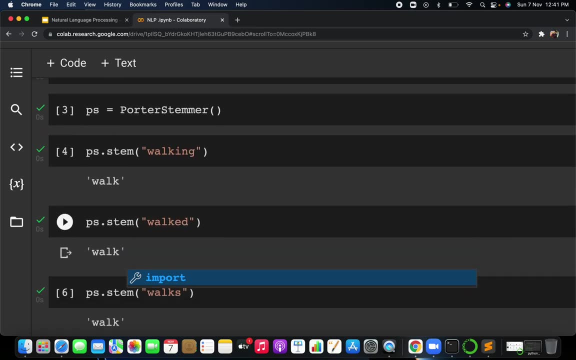 to use about this? uh, then second thing is the lanchester streamer. okay, so then after for lanchester streamer, you can just import directly. you can just import, you can already. we have just imported there. even you can just go there from nltk dot stem. 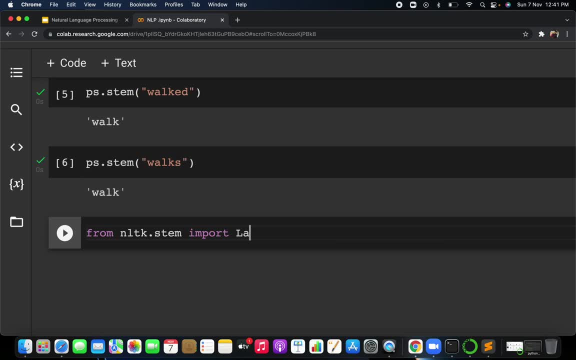 okay, import lanchester lanchester streamer. okay, just import this one and make the object of that. i'm just writing lanchester ls. okay, just write and let's see, and then after that just run for that which particular streamer you are going to use. okay, so lanchester. 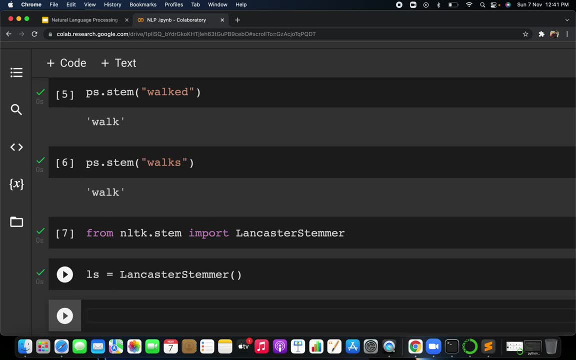 streamer is quite, really give it. give us somewhat more accuracy, you will. i will just make another video in that. i will just explain you what is the problem you are going to face in this particular, that is, the over stemming and the understanding. okay, so here in this video, you are only 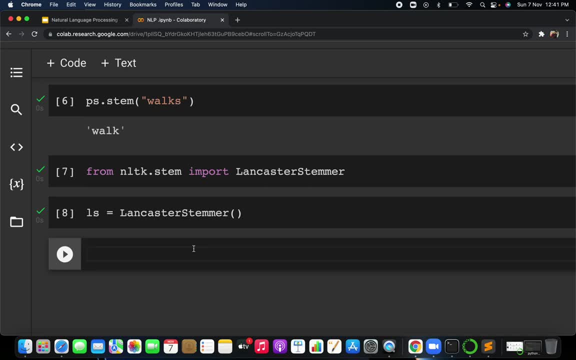 concentrating about the stemming and how, on which particular three type of stemming, you have to implement that particular. okay, that is the really basic concept and we have already. we have seen, for the protest streamer, then you are going for the lanchester streamer. okay, so lanchester streamer. 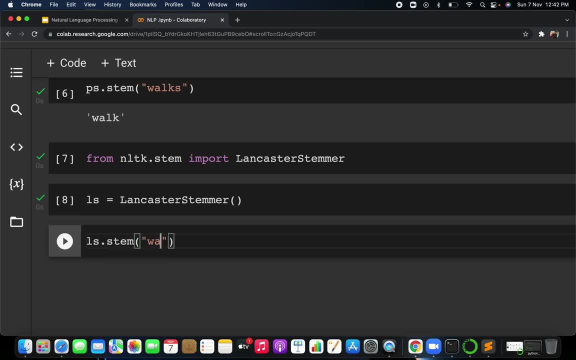 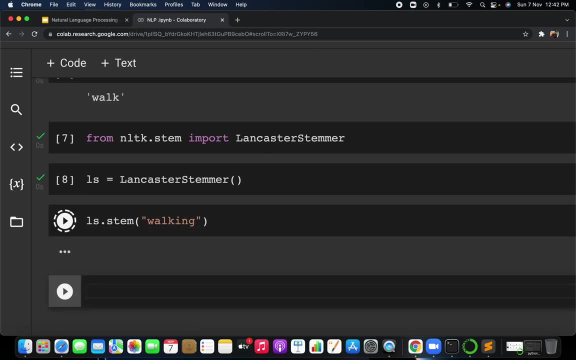 you can just write the same thing, okay. even you are just, uh, going for the walking. also, you are just seeing for the walking, so see, uh, okay, i have just given the okay, okay, and then after, if you are going to the stemming of the walk, okay, so i'm just showing. 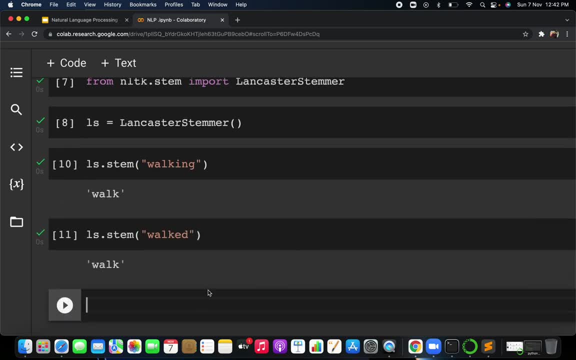 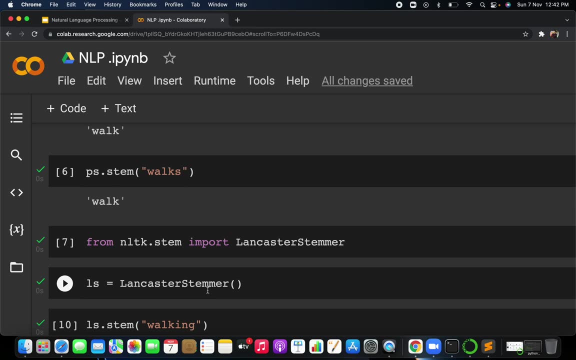 it will. just everyone will give the same the walk, you the walk, and then so on. okay, so again, why we are not using? so what estimates? really, really famous as compared to the lanchester streamer? okay, but there is also some drawback of stemming that we are going to see in after this. 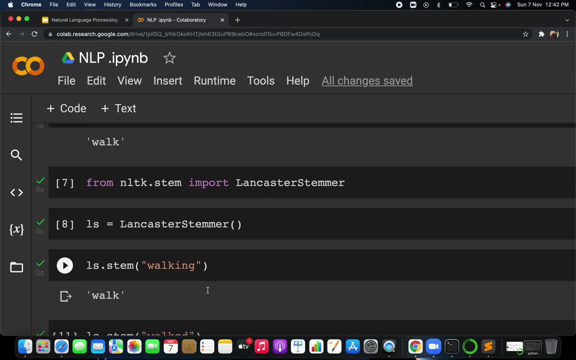 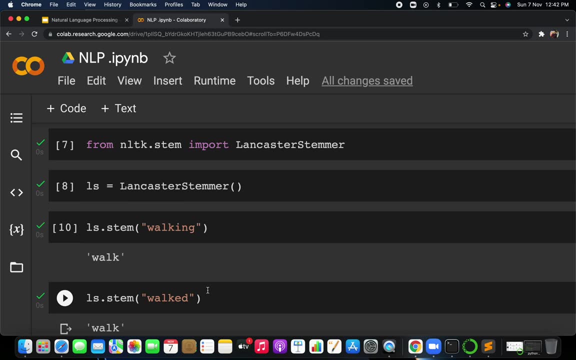 uh, this video after competition of these three technique. okay, so you are clear with the porter streamer, you are clear with the lanchester streamer: how to import and how to use the lanchester streamer to you, you, you can use this particular steamer steaming technique. okay, the last one is the 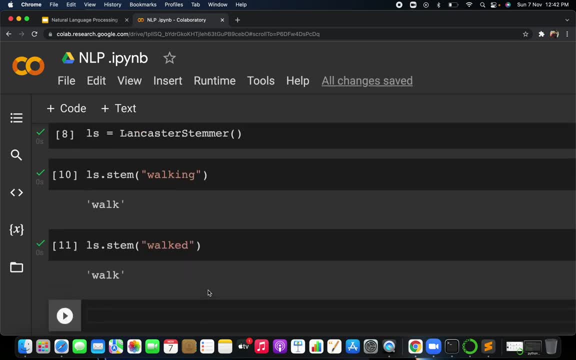 snowball steamer. okay, so snowball steamer is really an advanced version of lanchester steamer. okay, so they have first discovered the portal streamer, and it was, it is, and then, after that, then gave move to the lanchester steamer, the someone they have just discovered, lanchester. 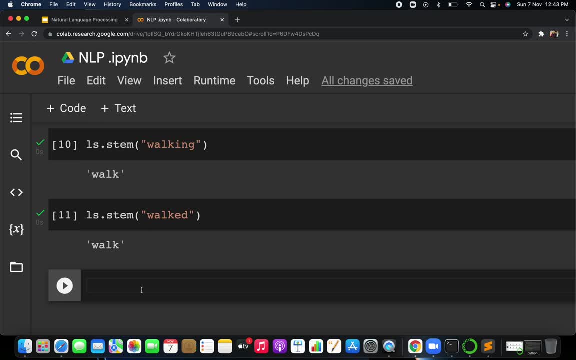 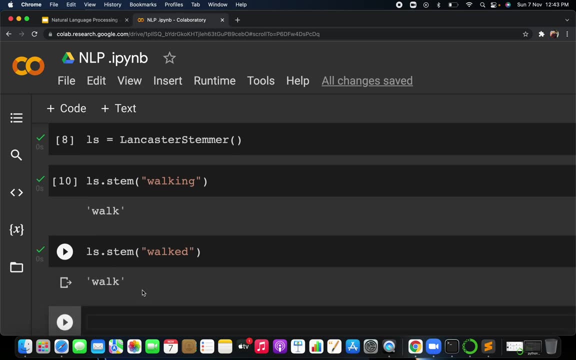 steamer and then, after they just go for the snowball, that is the advanced version of the lanchester steamer. okay, and the third thing is that why i have explained you in the theory part, that is, simply chop up the last word. okay, that is the ing or ed. okay, suffix or prefix. okay. 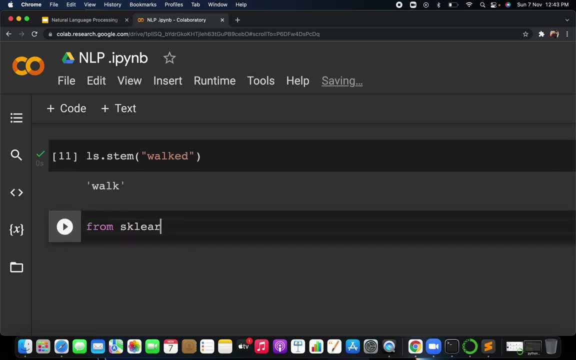 then after for the importing the snowball, you can just write the same. okay, why, i'm just writing a scale up. okay, you can just write: from nltk dot steam, import what you are going to import. you are going to import only snowball. okay, snowball, that's a snowball streamer. then just make the. 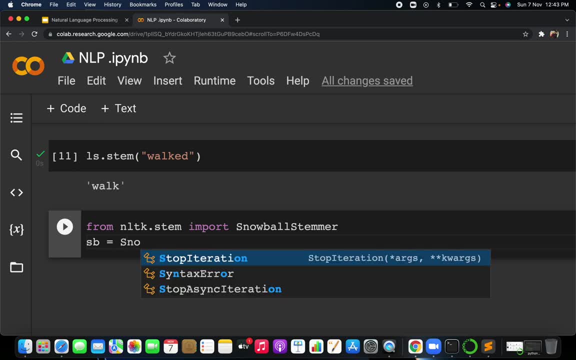 object of that snowball and then, after you are going to see, first of all run this library whether it is giving me error or not, yeah, it's fine. then after what you are going to do, so i'm making the object of that. okay, that's it. it's like the same thing what you are going to. 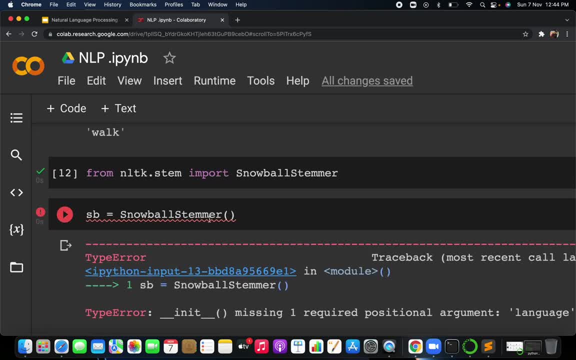 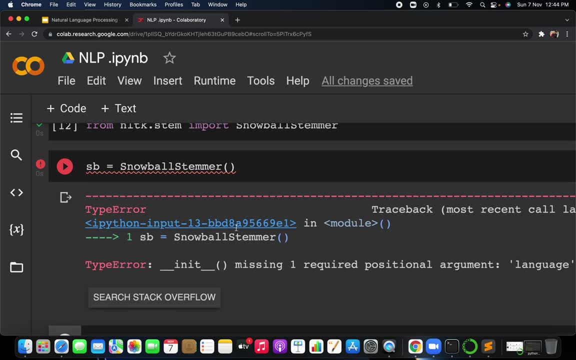 use. i'm, you, can. it depends upon you which particular type of technique you are going to use. okay, so i just, if it is giving me some mistake, we are going to see lanchester steamer, snowball steamer. okay, okay, okay, the why you have just, uh, just. 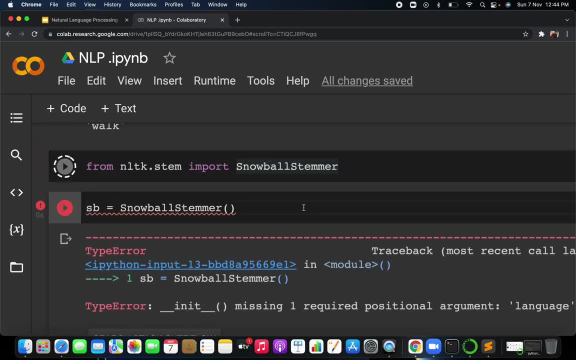 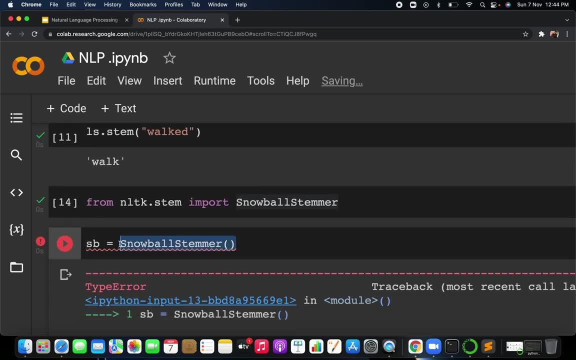 creating this error because whenever you are just running this one, okay, you have to. if i already have said that it is the advanced version of lanchester streamer, okay, so how you are going to use, you have to just call this particle lanchester, lanchester streamer, this particular lanchester streamer, you. 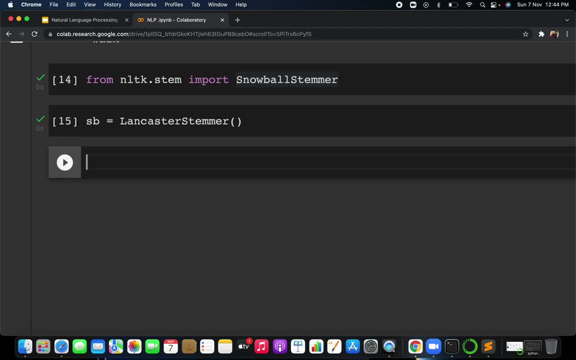 have to call, then after that, what you have to. you have to write which particular thing you want to go. okay, and even one thing you can just try. okay, you can just try. uh, you can just try with the snowball wall, and here just keep the one parameter that only for the english i'm going to use, okay, 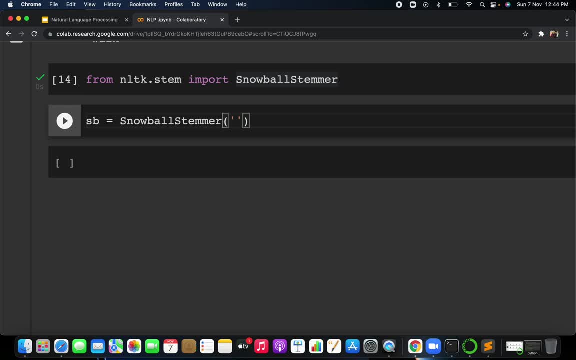 so snowball is really advanced version of the lanchester and the portal. so here you have to specify this. take one parameter: whether you are going to stemming this particular what. is it related to the english, or it is related to the french, or it is related to the other language? okay, 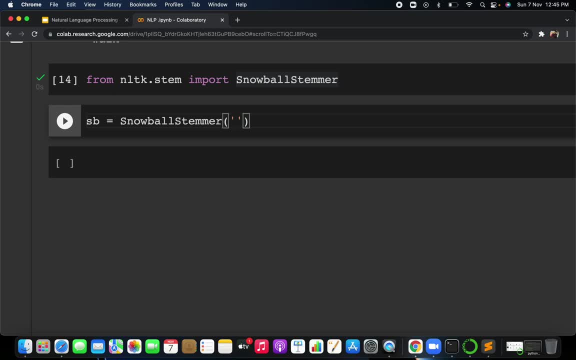 you have to specify which particular language you want to. going for the stemming, okay, whether, if you are choosing the english, okay, so you can just write the english word. if you are choosing the phrase, you have to write the french word, okay, you can just write the english. i'm going for the. 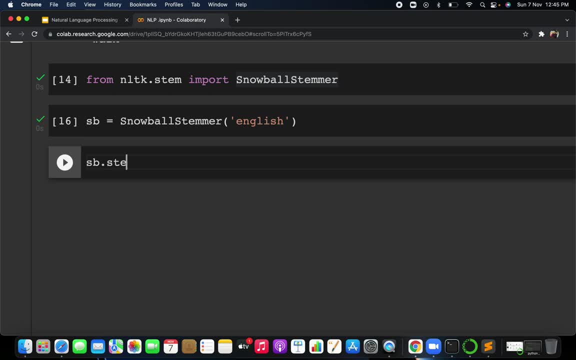 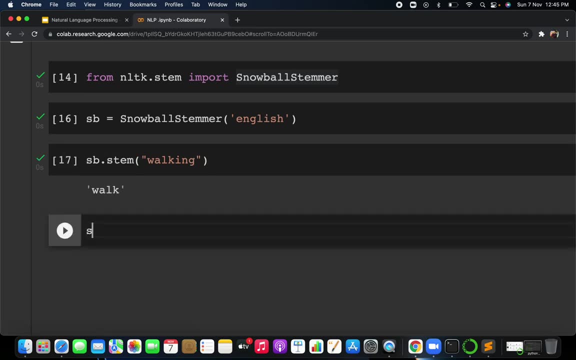 english. okay, now it will not give. then after you can just write the same, every concept is like same, okay, and just write the walking: okay, see, okay, so it. and then after walk also you can just see. you have just given a similar example, so you are able to see why. to pass here, though, you can just 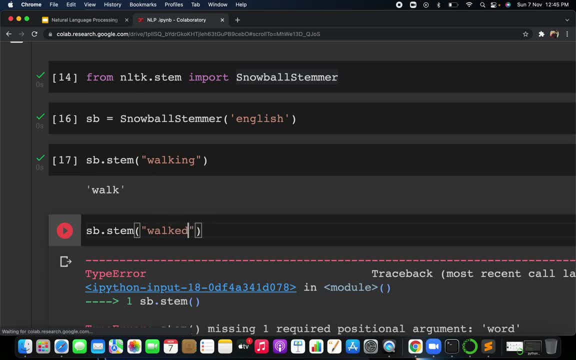 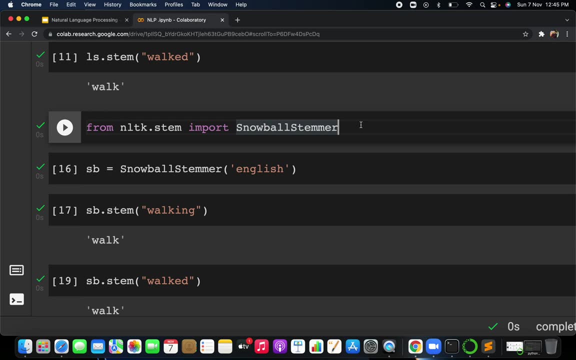 fast walked. okay, so see, it will give you walk. okay, so i don't think so you have problem, you. so you are able to see that every three technique they have used. but you will say why we are going for snowball. that is advanced mention, so there are some cases, okay. so in the next video we will see. 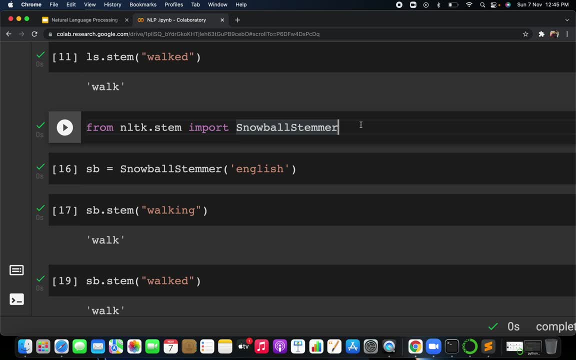 what was the problem of related to the stemming? okay, you uh the problem that has related to the stemming and how there was two type of problem you will face in the stemming, that is, the understand understanding and over stemming. okay, so i will explain you this concept in the next video and